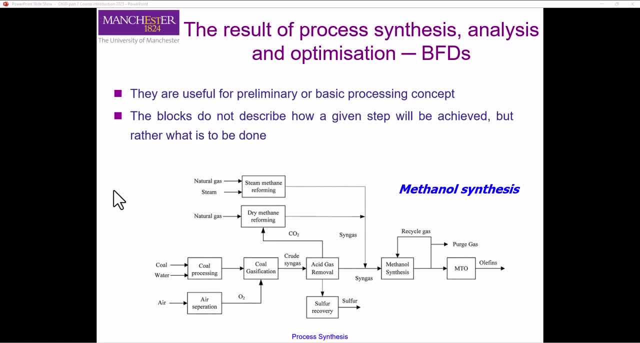 At the inception of any industrial process, engineers and designers rely on flowsheets to conceptualize their ideas. These early-stage flowsheets, such as block flow diagrams or VFDs, help to visualize the overall process layout, what are the major unit operations and how materials flow between these unit operations. 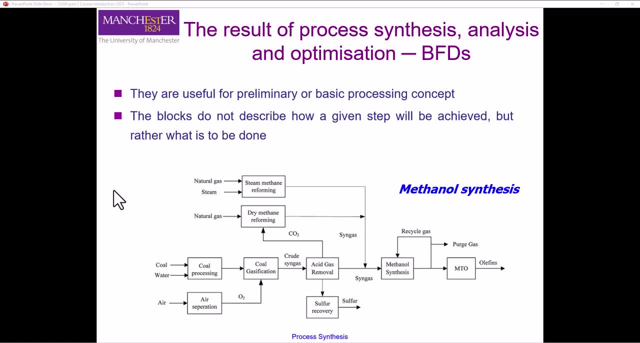 So you can think of them as the blueprint of your entire project. In block flow diagrams, the blocks do not disappear. They do not describe how a given step will be achieved, but rather what is done. For example, here you have the block flow diagram of methanol synthesis. 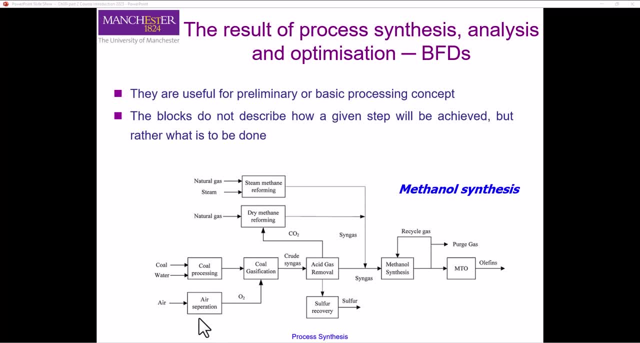 If you look here, the first block says air separation. So that means that it is telling you that air needs to be separated from air to oxygen, but it doesn't state how this separation will be achieved. Similarly, here this block says that steam methane reforming. 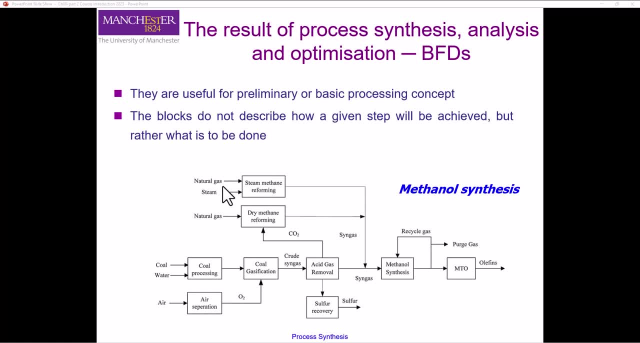 so it means that the natural gas needs to be converted into syngas, but it doesn't say what kind of reactor or system you are going to use for this steam reforming. So this gives you a very basic blueprint of the process, just explaining what are the steps in this process, without giving any detail. 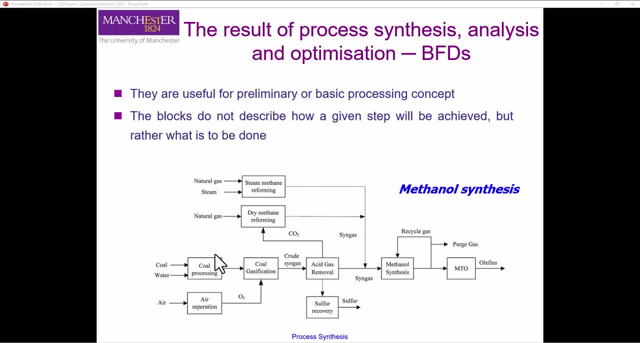 what that step, how we are going to achieve that step. So, in summary, block flow diagrams provide as the blueprint of the whole process and help us grasp the bigger picture of the process. Now let's look at what are process flow diagrams. 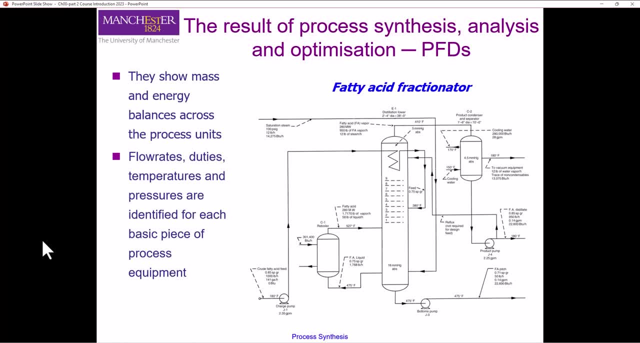 So, as the project progress, process flow diagrams come into play. These detailed flow sheets provide a comprehensive view of the process. These are step up in detail from BFD and PFDs, or process flow diagrams offer more granularity by detailing individual process units. 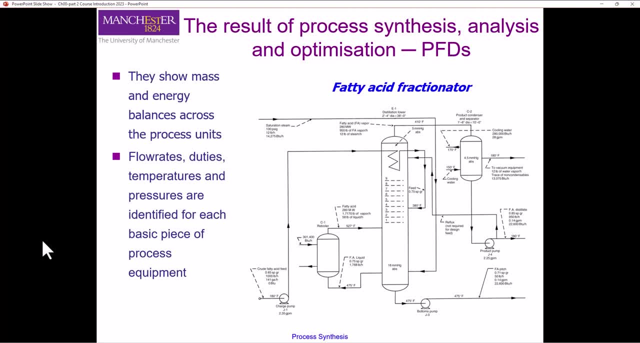 They show the flow of material, energy and utilities and how they are connected. And process flow diagrams are crucial for a deeper understanding of the process. For example, you can see here the process flow diagram of fatty acid fractionator And you can see that much more detail is visible. 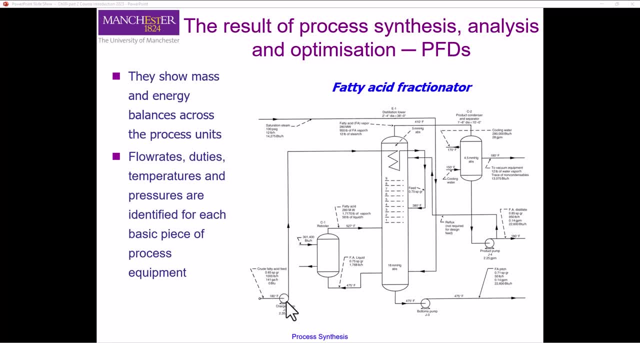 On this, on the, on this flow sheet. So here, for example, you have a pump and it tells you, for example, what are the flow rates or conditions of the of the feed, at what temperature it is and what is the power or duty of this pump. 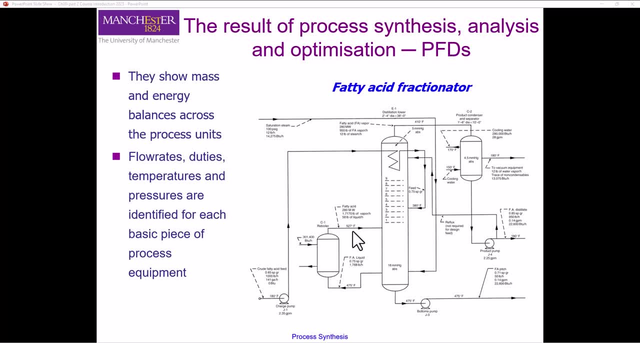 And then, similarly, for each equipment and each stream, you have much more information available to you, telling you the type of the system or the type of the stream, its temperature and pressure conditions, And its phase as well. OK, Next we have piping and implementation diagram, or in short, P&IDs. 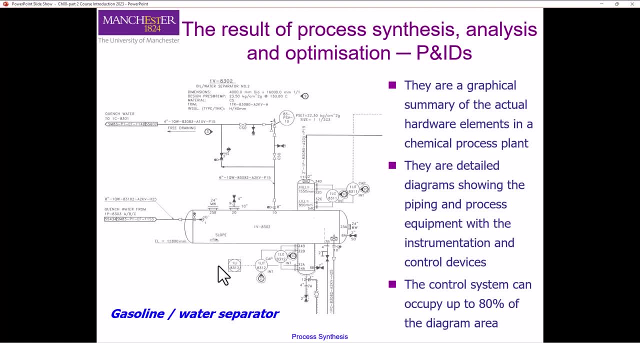 P&IDs detail the piping instruments and control within each unit And they help engineers and operators understand how equipment is interconnected. OK, So P&IDs are indispensable for safety and operation And also for regulatory compliance of our process. And here you can see a section of gasoline water separator. 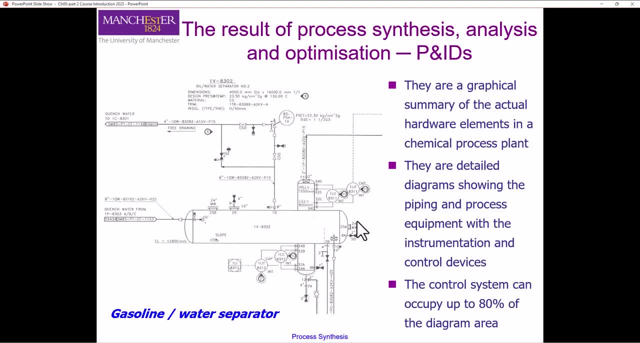 for example here, And so this is one unit that you will see in process flow diagram, And the rest of it is just all about piping and control. OK, So sometimes 80% of your piping and instrumentation diagram is just the control and piping system. 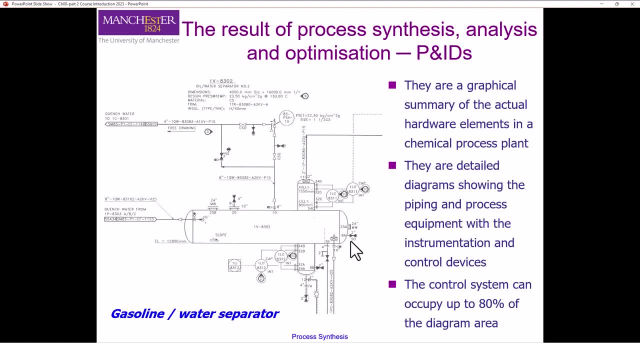 OK, Here, for example, you have this separator as a process unit And then you have a lot of valves that are controlling what is going to come in to the system or what is going to come out, And if, for example, for some reason, the outlet valve shuts, 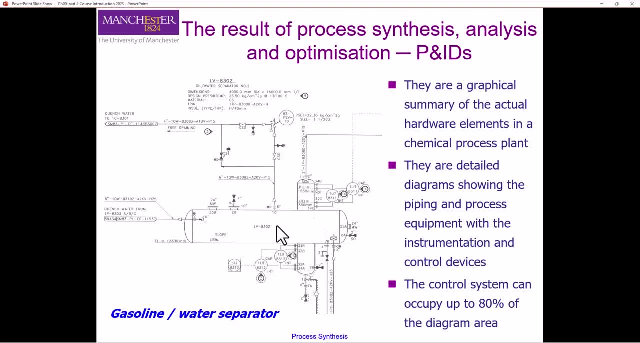 how you are going to ensure that the equipment is not going to blow up. OK, And in that case you have, for example, safety pressure valves in case, if the valve is not working, the safety pressure valve is going to open and release all the gas. 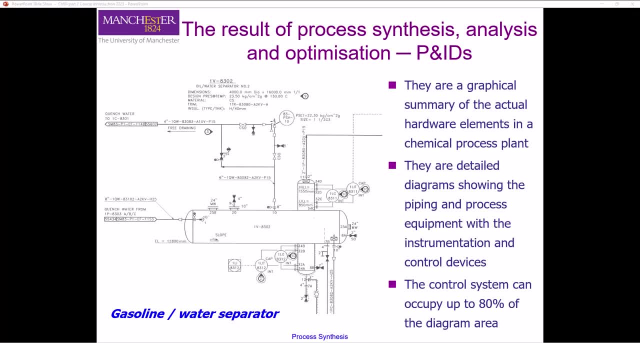 or liquid to the environment. So in your next semester, when you will do your design project, you will need to provide a process flow diagram and a piping and instrumentation diagram. OK, So in the process flow diagram, as I said that you will list all your equipments, how they are connected. 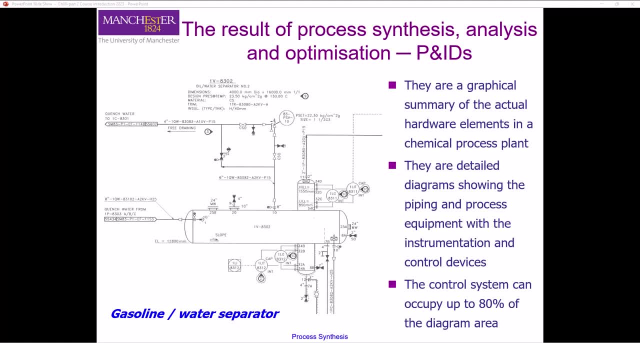 And for each equipment and for each stream you need to provide the temperature, pressure and flow rate conditions. And then you have the process and flow diagram where for each equipment that you show on your process flow diagram, you have to devise a control strategy. 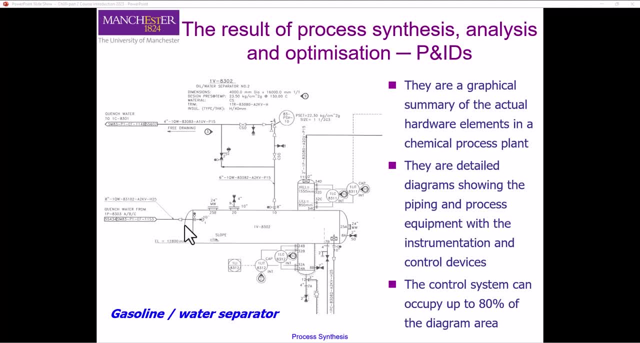 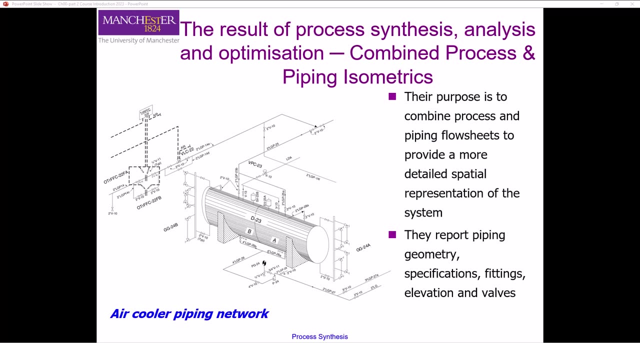 or how you will ensure that the process runs smoothly and also it's safe to operate. OK, These are the two pieces of information that you need to provide in the form of flow sheets in your design project. Now let's have a look at combined process and piping: isometric diagrams. 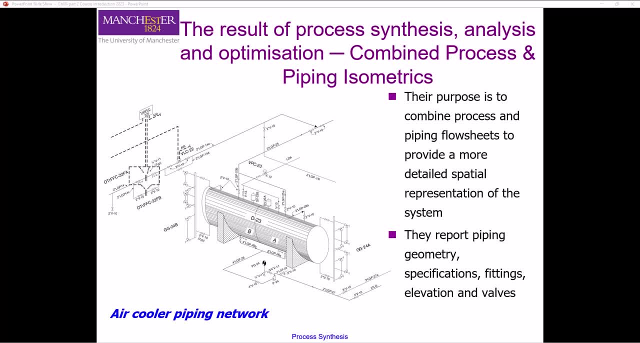 And these diagrams provide a more detailed view of the process. So isometrics provide three-dimensional representation of piping and fittings and they help with accurate material takeoffs and construction planning. OK, So that you can see that, what is the exact length of? 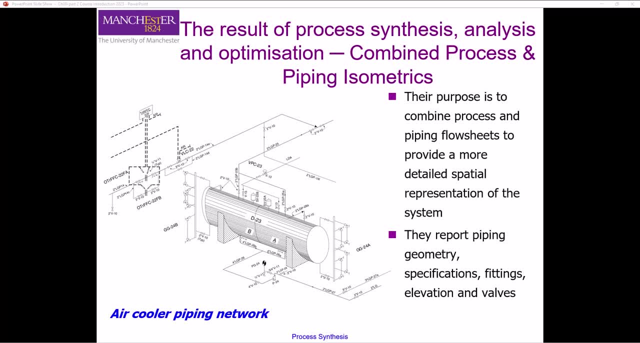 for example, a pipe, that you need to connect different equipment. as such, you can actually reduce wastage and reduce cost overruns. So isometrics are valuable during construction phase. Contractors and workers can use them as visual guides to ensure that the installation aligns with the design. 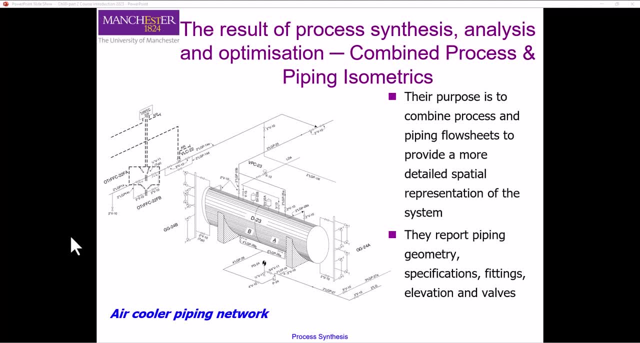 OK, So even this simplified version of this isometric diagram actually can help you reduce errors when you are constructing a process, And these isometrics are essential part of the documentation package for any industrial facility. OK, So they provide a clear record of as-built system. 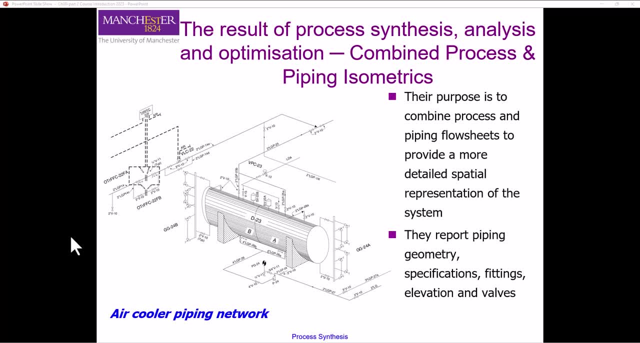 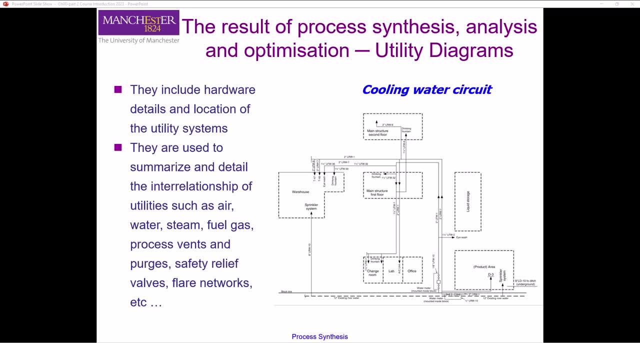 aiding the future modification, expansions and regulatory audits. Now let's have a look at what are utility diagrams. So utility diagrams include the information about the hardware details and location of utility systems. OK, For example, here in the figure you can see that this is a cooling water circuit. 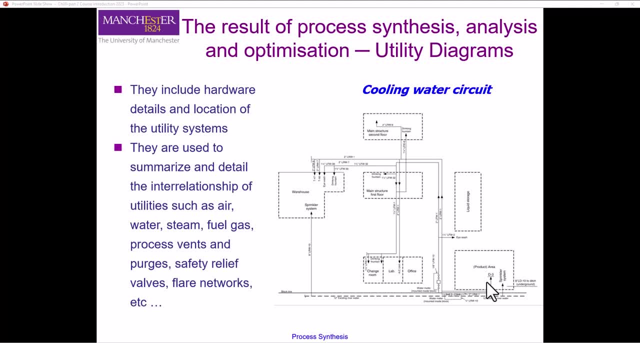 OK, So this is showing that how cooling water is provided throughout this process plant. So here, for example, you have warehouse where you have a sprinkler system, Then you have the product area, Then you have the liquid storage And then you have, for example, 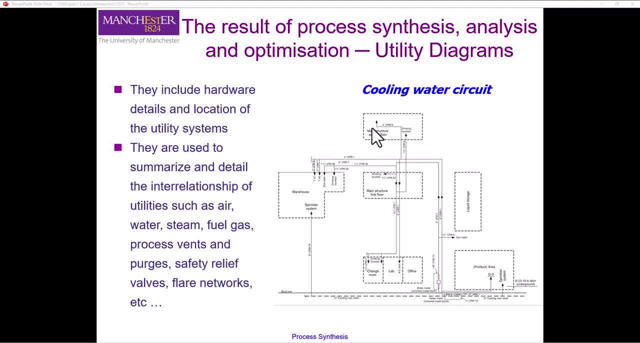 here you have the main structure of the building. OK, So how the cooling water is distributed throughout this facility is shown here, and what kind of piping is required or what are the dimensions of these pipes. All information is available here. So utility diagram in its simplicity.